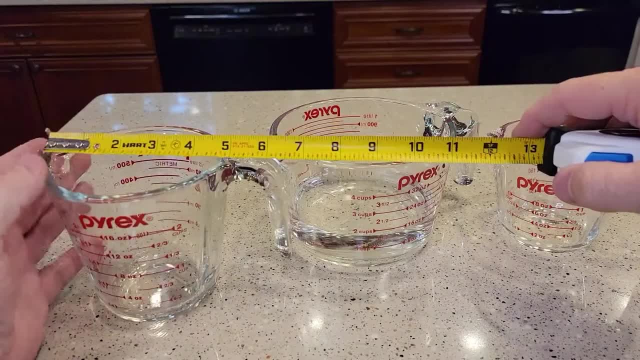 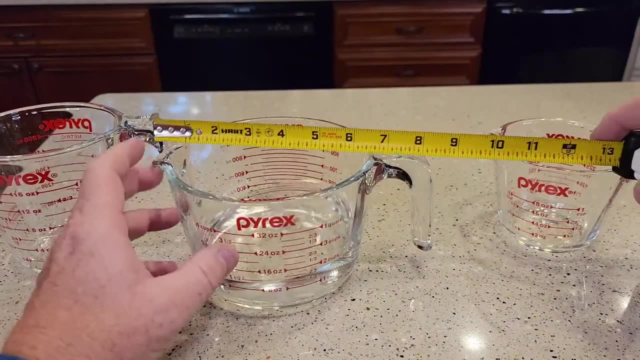 Okay, so let's go over measurements. You know the two cup. you know the cup size is about four and a half, but with the handles almost seven. The four cup, all the way to the end of the handle, is almost eight and a half. 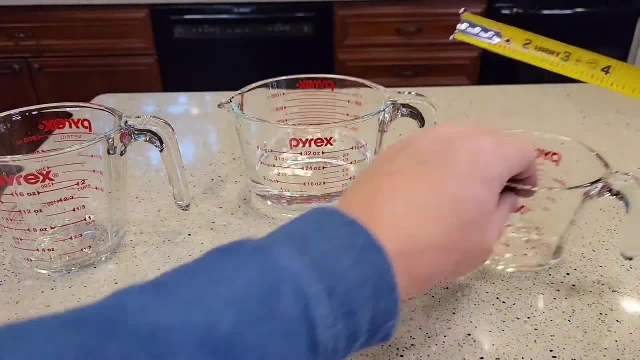 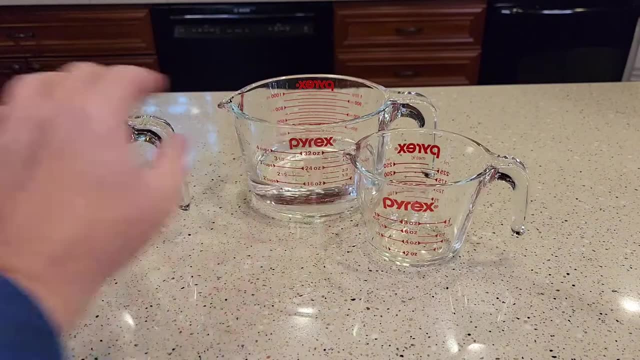 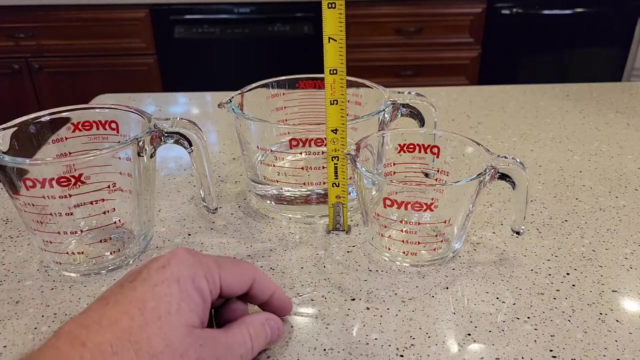 Inside is just five and a half, And then the smallest one, from spout to handle six, inside is about four. Now, all of these are relatively surprisingly. the two cup is the tallest, at four and a half, The four cup is about four and a quarter and the one cup is about three and a half. 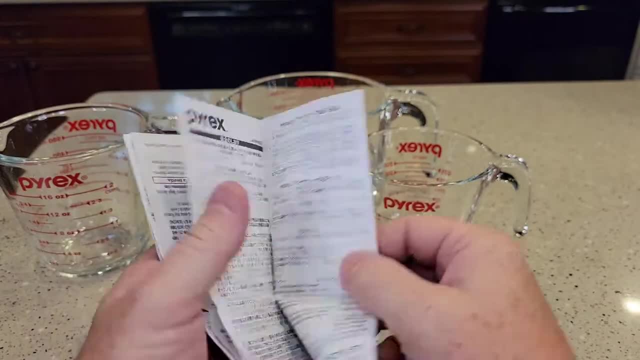 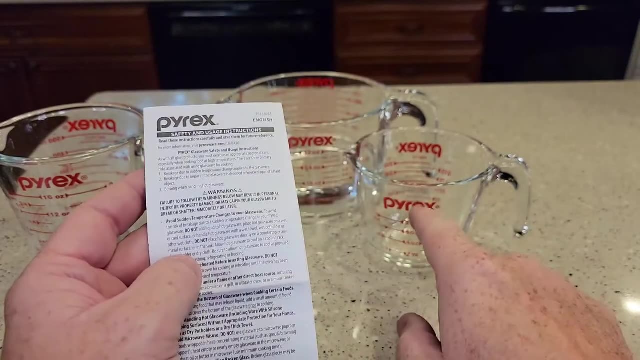 So hidden in the box there is safety precautions kind of a manual. This does warn about sudden temperature changes. Okay, Like if you've got it filled with ice and then you pour hot, scalding hot water in there. it says it could crack. 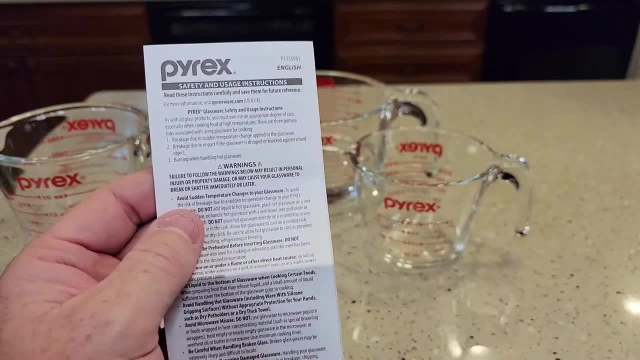 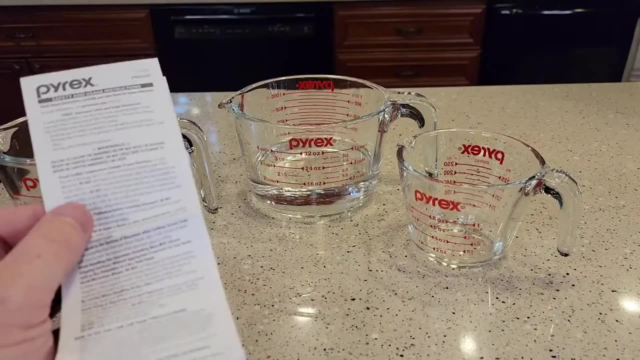 And if you drop it it could, or knock it hard it could. So it talks about the heat could transfer to the handle, so your handle don't get burnt there. And it does say that they're all dishwasher safe. Okay, so I got some water in it. 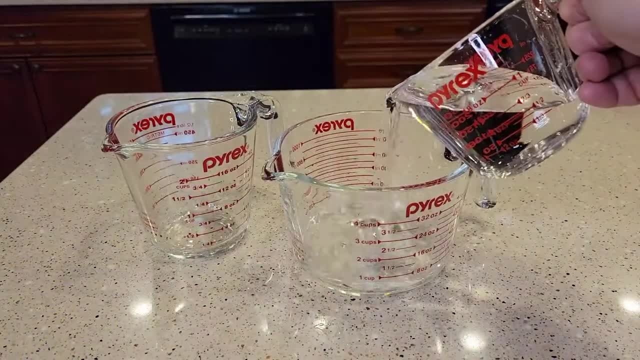 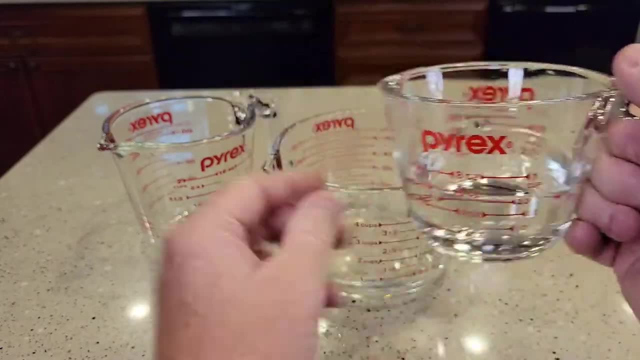 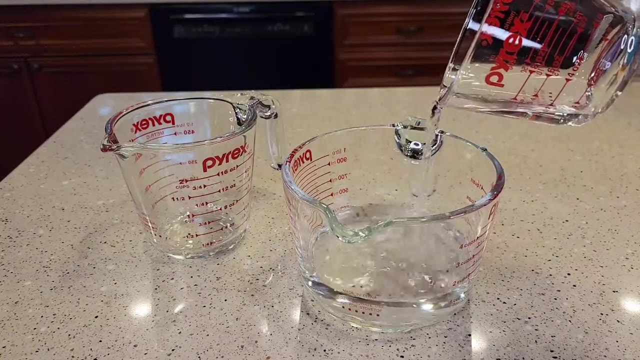 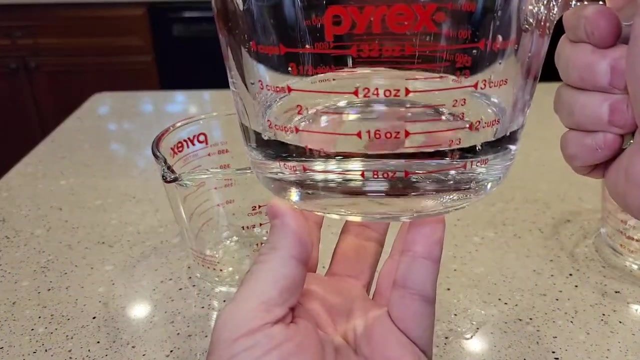 Let's play around, Let's see how it pours. Okay, I didn't go too fast, but it's Easy to see the markings And let's do pouring. Yeah, Let's try the big one. Yeah, easy to see markings. 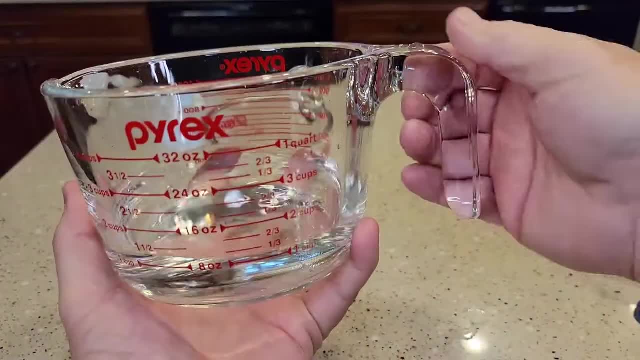 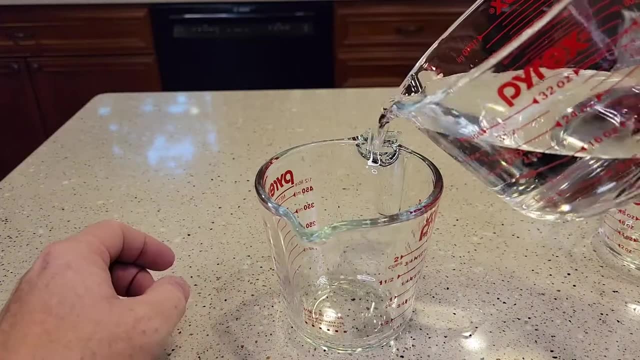 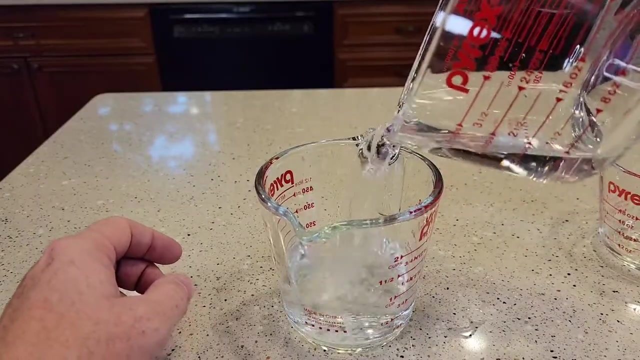 Now I do find, I do find this part to be kind of slippery, So be careful. This part is kind of slippery. Let's see how it pours. Okay, Let's go slow. Yeah pours, okay, I'm having problems there at the first. 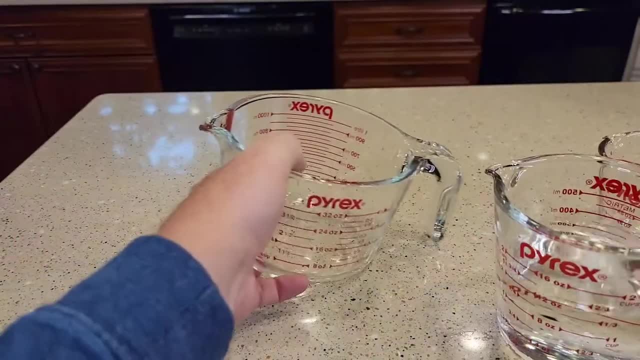 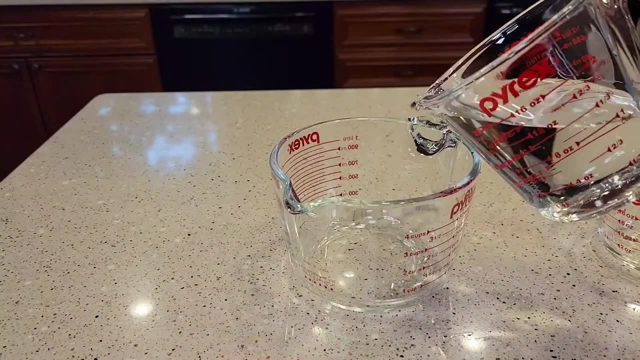 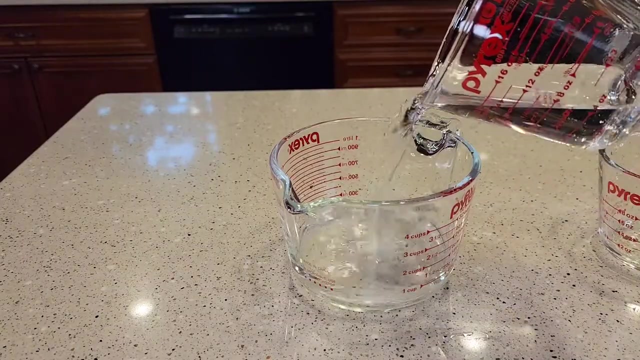 This is the perfect size. right here, The two cup one is like the perfect size. Yeah, it also seems like it pours the best, Because you're able to control it better. Okay, Yeah, I like these. Okay, Yeah, I like these.